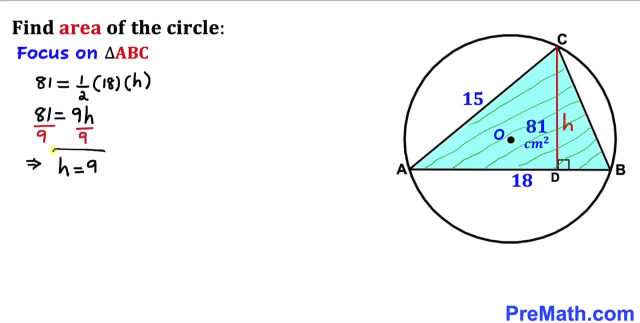 our H value turns out to be 9 centimetre. So thus our height H turns out to be 9 centimetre. And now let's focus on this right triangle, ADC, whose side lengths are 9 and this longest leg is 15.. And now we are going to calculate this side length, AD. and now let's 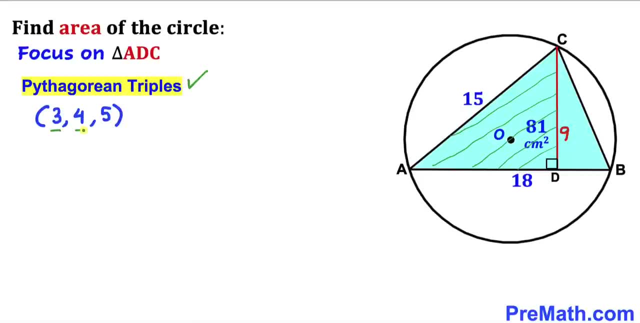 recall, the got a Pataeagrian triplez of 11 minus 2 times H. And now let's add that the long s and z are 3,, 4 and 5. Let's go ahead and multiply all these numbers by 3.. Then, after a multiplication of 3, 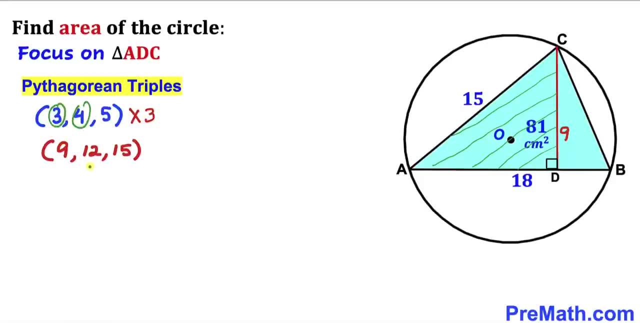 this, 3 is going to become 9, 4 is going to become 12 and 5 is going to become 15.. So, in our case, we got this 9 and this is 15.. So, therefore, this unknown side length, AD is going to be 12. 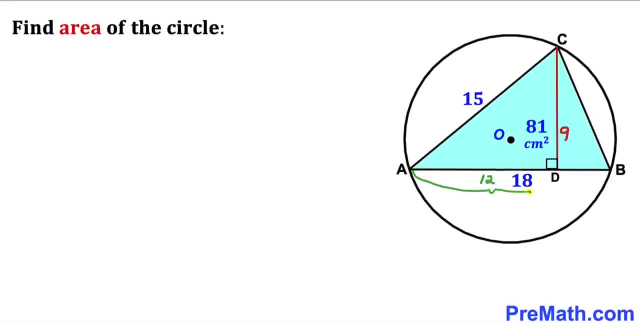 centimeter. And now we know that this whole chord AB is 18.. This length is 12.. So, therefore, this length BD is going to be 18 minus 12 is going to give us 6 centimeter. And here's our next step: I have drawn this diameter CE that passes through this center out, And then I have 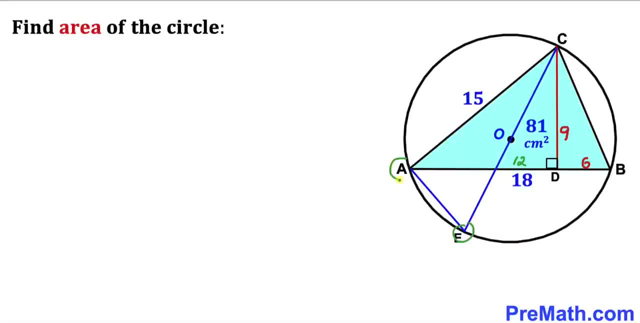 connected this point E with this point B, And then I have connected this point B with this point E, And then I have connected this point E with this point B, And then I have connected this point E with this point E, As you can see. And now let's recall the Thales theorem. According to this theorem, if E, A and C are: 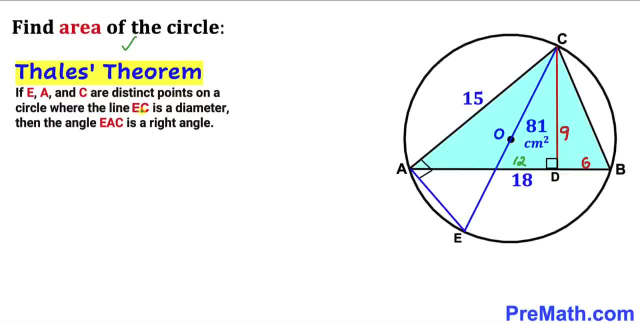 three distinct point on the circle. where the line EC is a diameter, then the angle EAC is a right angle. As you can see in our diagram, we got CAE, three points on this circle, and this EC is a. this angle is 90 degrees. So therefore we conclude that this triangle, EAC, is a right triangle. And now let's recall: 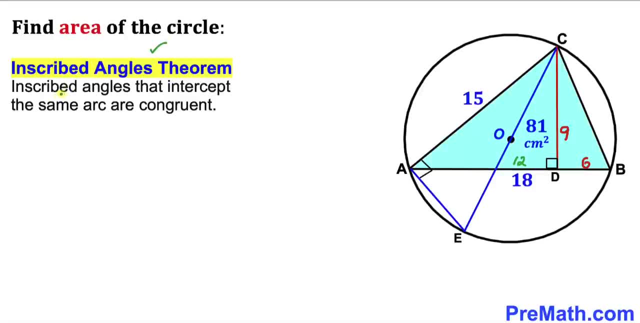 inscribed angles theorem. According to this theorem, inscribed angle that intercept the very same arc are congruent. And now let's focus on these two angles, Angle E and this angle B, And both of these angles make this very same arc, as you can see. So therefore, we conclude that these angle AEC and this angle DBC are congruent. 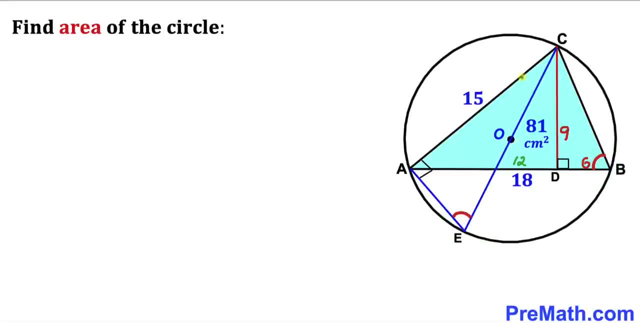 And, furthermore, this angle in this triangle, EAC and this another angle in this triangle, BDC, are congruent as well, Since these other angle is congruent And this other angle in this triangle is congruent, photo shown And now we are going to solve for this sin x, y Door, And now we are going to have a proportion in these two similar triangles. 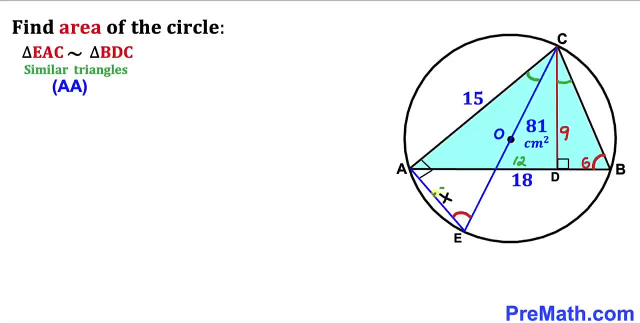 So, therefore, we conclude that this triangle EAC is a right angle. As you can see, if we compare these angles, EAC and this, the ones that are congruent, In other words, the ratio of x and 15 is going to be equal to the ratio of 6 and 9.. 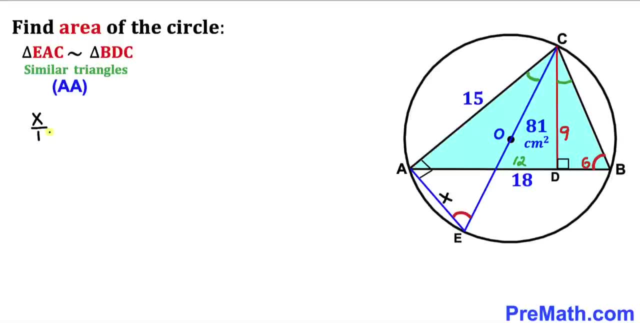 So, therefore, let me go ahead and write down x divided by 15 equal to 6 divided by 9.. Let me go ahead and multiply both sides by 15 to isolate x, And here 15 and 15 is gone. So x turns out to be equal to 6 times 15 is 90.. 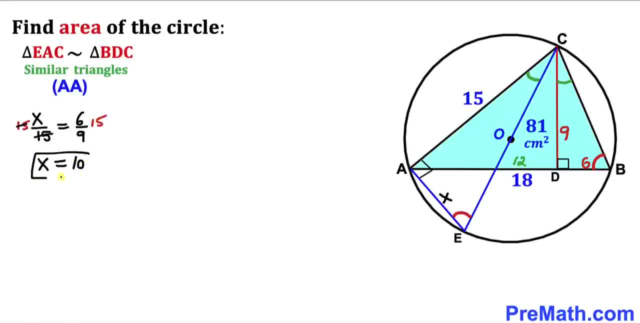 90 divided by 9 is going to give us 10 centimeter. So, therefore, this length AE turns out to be 10 centimeter. And here's our next step. Let's focus on this right triangle, EAC, whose side lengths are 15 and 10.. 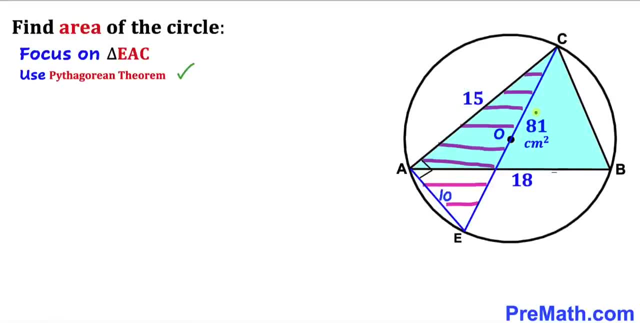 We are going to use the Pythagorean theorem to calculate this side length EC. And here's our Pythagorean theorem: A square plus B square equal to C square. Let me go ahead and call our longest leg as our side C. I'm going to call this side A and this side lowercase b. 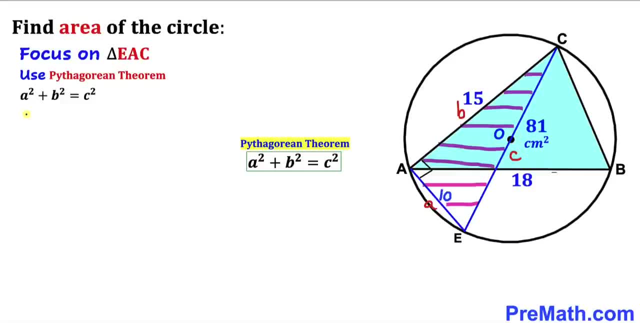 So let's go ahead and fill in the blanks in this Pythagorean formula A, in our case 10.. So it's going to become 10 square plus B is 15 square equal to C square. So therefore our C square value turns out to be 325.. 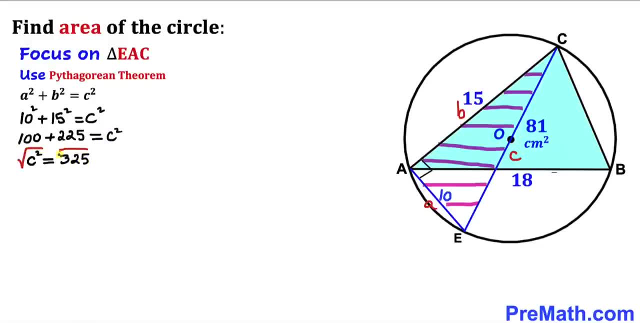 Let me go ahead and undo this square by taking a square root on both sides. So therefore our length C turns out to be square root of 325.. So thus we can see that this EC length turns out to be square root of 325.. 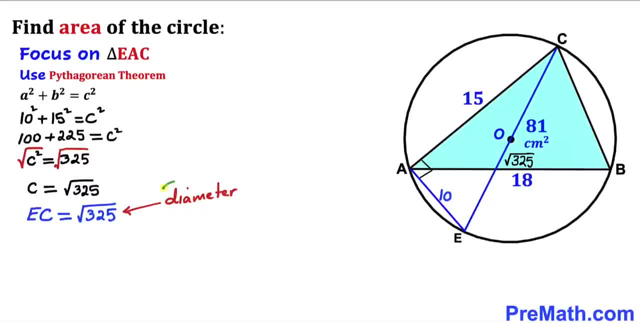 As you can see, As you can see, As you can see over here, And that is also our diameter. So, therefore, the radius of this circle is going to be half of this diameter. Let me go ahead and label: radius R equals to square root of 325 divided by 2.. 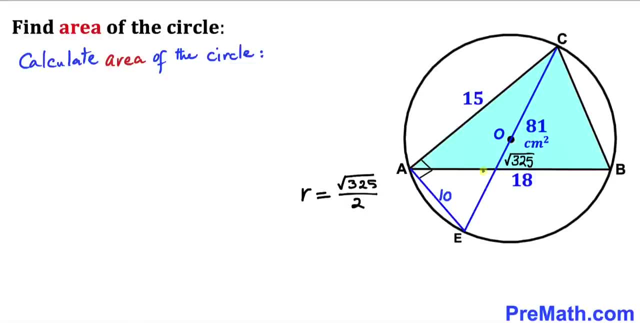 And here's our final step. Let's go ahead and calculate the area of this circle. And now let's recall the area of a circle formula. Area equals to pi. And here's the area of a circle formula. And here's the area of a circle formula. 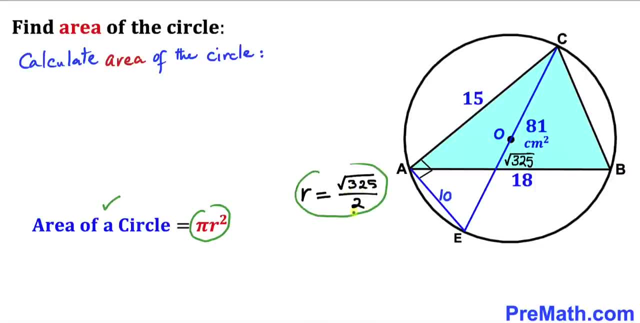 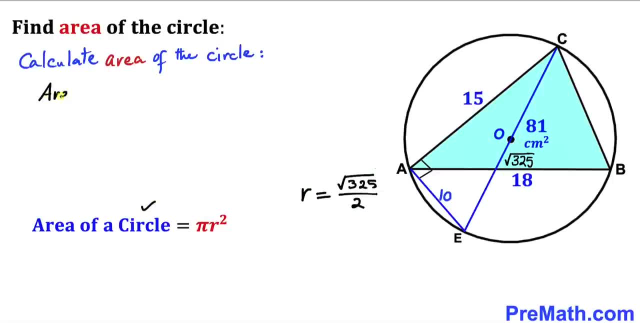 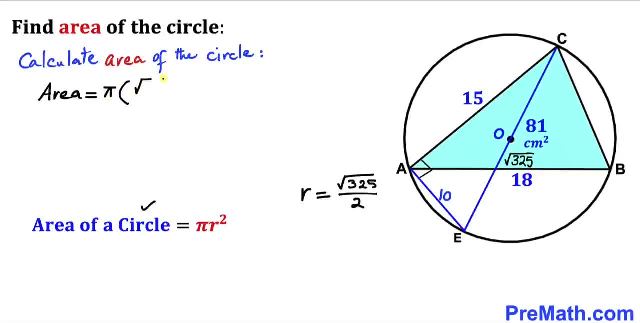 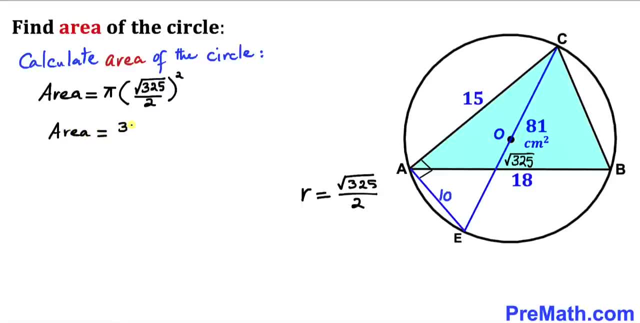 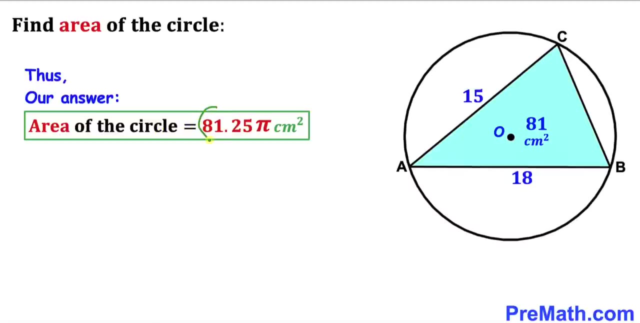 this circle is going to be 325 pi divided by 4, and that is going to be equal to 81.25 pi, so thus the area of this circle turns out to be 81.25 by centimeter square. thanks for watching and please don't forget to subscribe to. 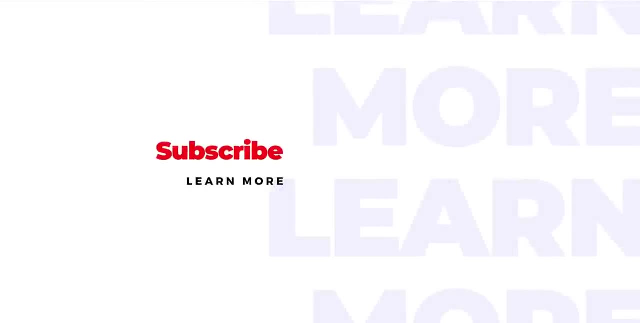 my channel for more exciting videos. bye.